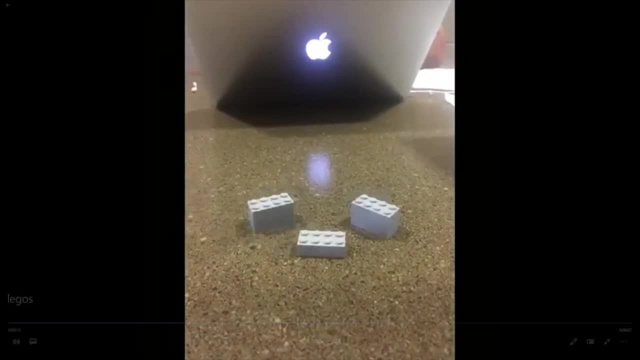 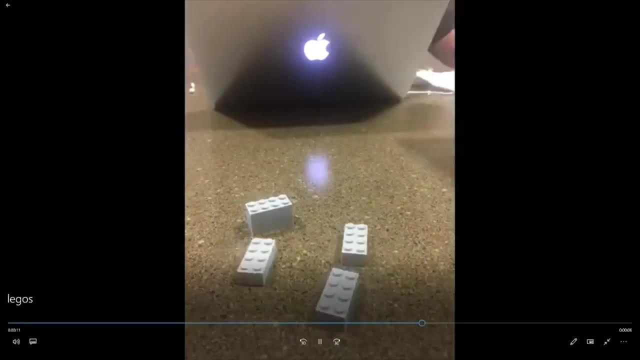 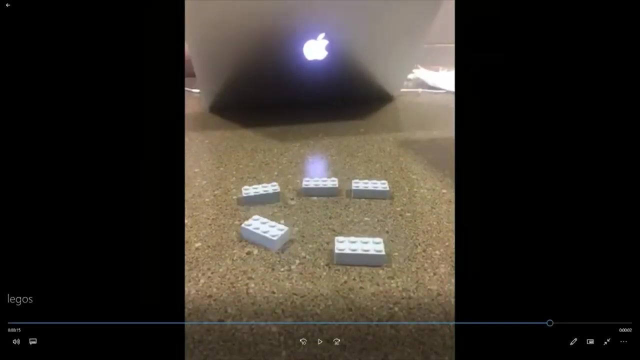 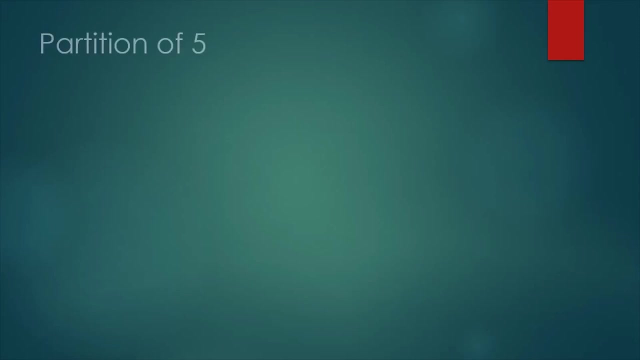 of 5.. three plus two, two plus two plus one, two plus one plus one plus one and finally five ones to make the seventh partition for the number five. To go over what we just did in lego form, we will now demonstrate the partitions of five. 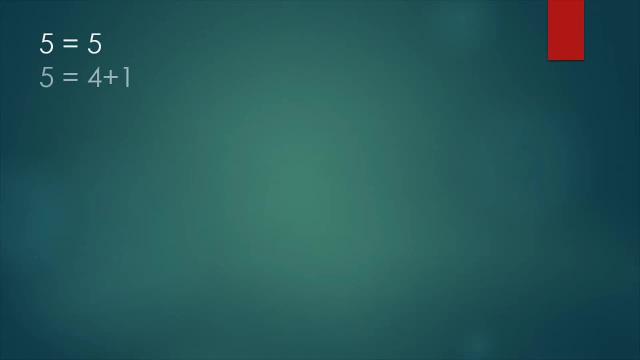 As you can see, five is a valid representation for a partition of five, along with four plus one, three plus two, three plus one plus one, two plus two plus one, two plus three ones, and then five ones, giving five a total number of seven. 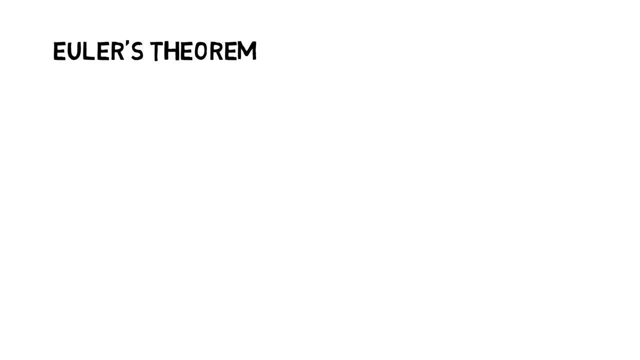 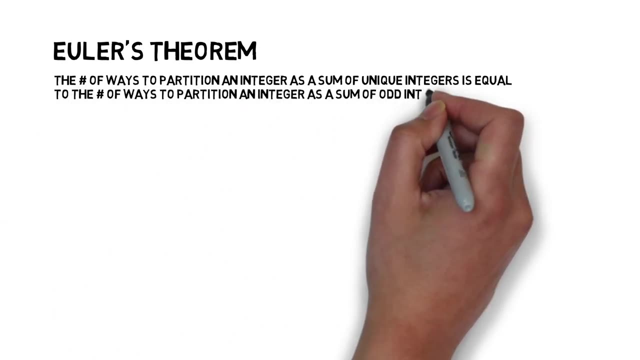 partitions. Now let's take a look at Euler's theorem. Euler's theorem states: the number of ways to partition an integer as a sum of unique integers is equal to the number of ways to partition that same integer as a sum of odd integers. For example, let's take a look at the partitions of five Of the partitions of: 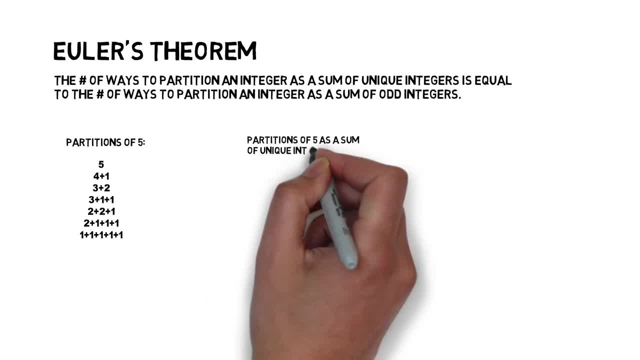 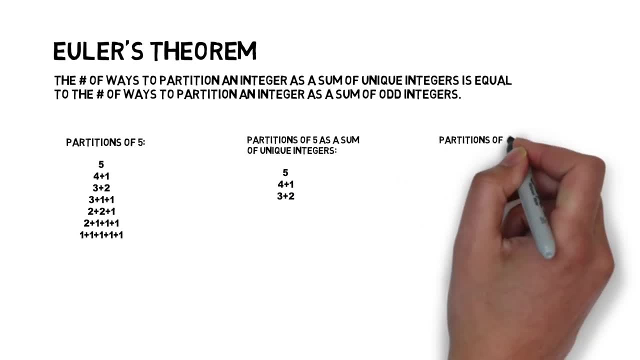 five. how many of them are a sum of unique integers? Well, we have three of them. We have five, four plus one and three plus two. Now, how many of the partitions are a sum of just odd integers? Well, we also have three of them. We have. 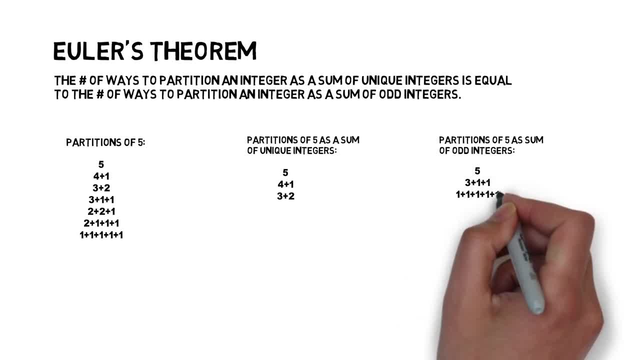 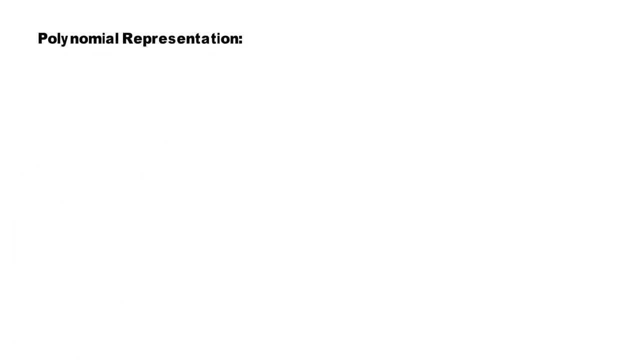 five, we have three plus one plus one and one plus one plus one plus one. Now Euler stated that we could represent the number of ways to partition an integer as a sum of unique integers with the following polynomial: one plus x times one plus x squared, times one plus x cubed, and so forth. 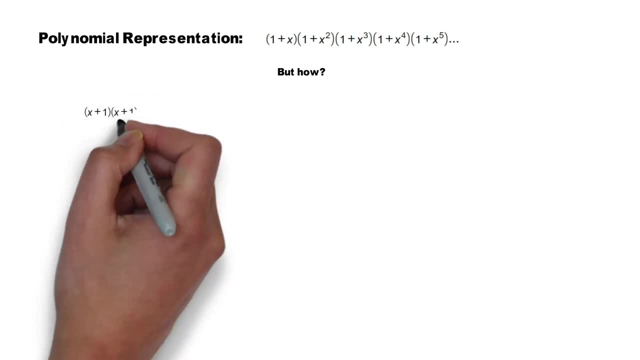 But how come? Well, let's take a look at this example: X plus one times one plus x plus one. If we FOIL that, we will get one x squared plus one x plus one x plus one, and if we simplify that, we will get one x squared plus two x plus one. 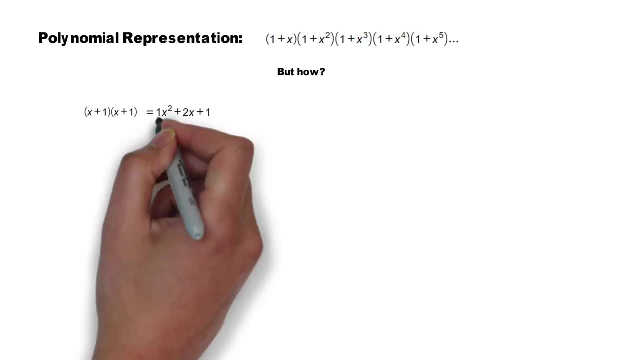 Well, if you look carefully, you you can see that the coefficients before each x represent how many ways we can get that type of x, For example, x squared. we can only get it once by multiplying the the two x's, but we can get x twice by multiplying the first x and the. 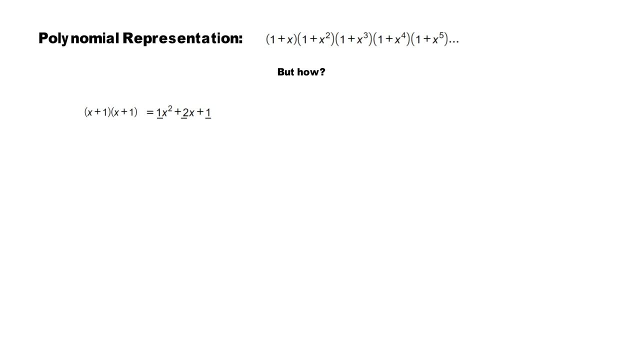 second number one, or multiplying the first number one and the second: x and one. we can get it by multiplying the two ones. Now let's take a look at this example: x plus one times x plus one times x plus one. We know we will get an x cubed here, so 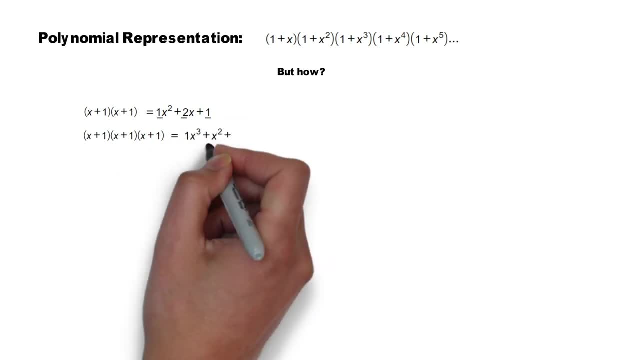 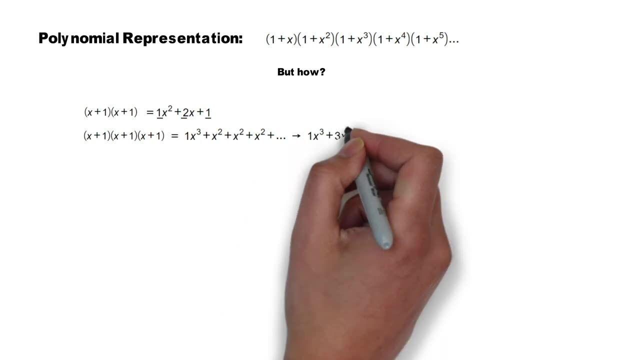 how many ways can we get x cubed here? Well, only once, by multiplying all the three x's. But how many times can we get x squared here? Well, we can get x squared by multiplying the first two x's and the last number one, or multiplying the last two x's and the first. 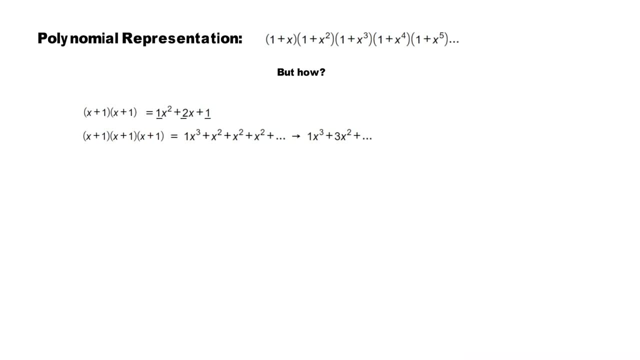 number one. or if we multiply the first x, the middle one and the last x, therefore, given us three ways of getting x squared. well, we can use this same idea when we expand the polynomial representation. How many ways can we get number one from here? 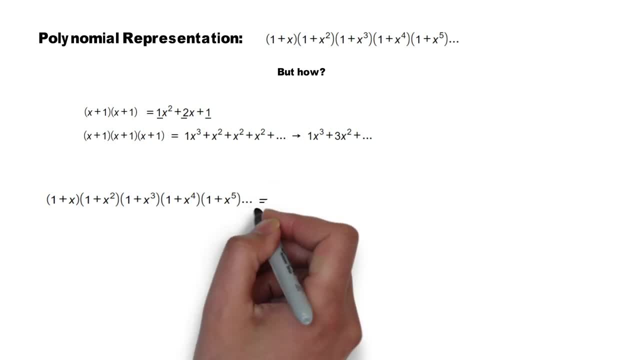 well, we can get it only one way, by multiplying all the number ones. How many ways can we get x from here? well, we can also get it once by multiplying the x from the first binomial and then the rest of the ones. How many ways can we get x squared? Well, we can get it only once, by multiplying. 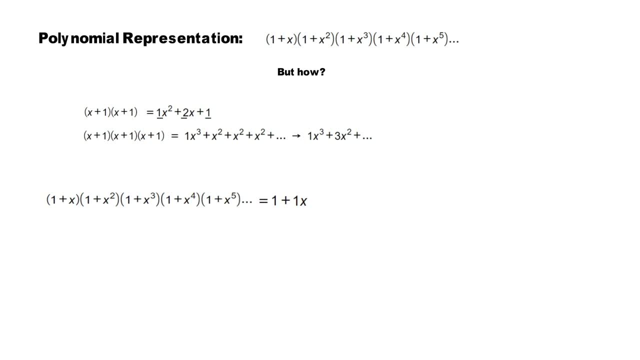 the x squared from the second binomial and then the rest of the ones. But how many times can we get x cubed here? Well, we can get it by multiplying the first x and the x squared, and then the rest of the ones, or the x cubed itself and the rest of the ones. 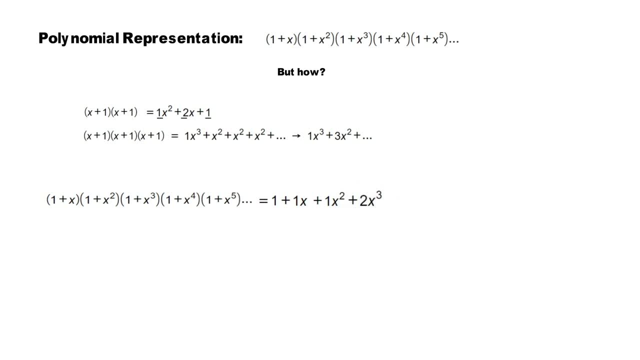 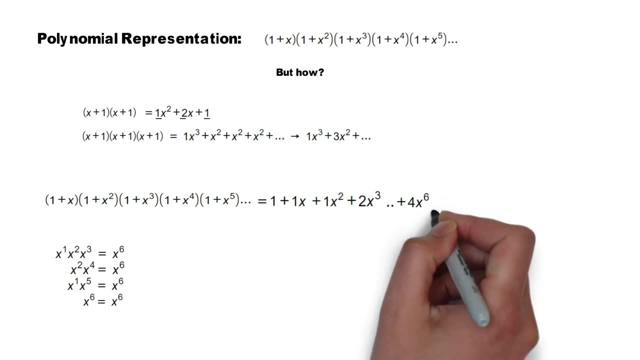 So twice, 2x cubed. But how many times can we, let's say, can we get x to the 6th? Well, we can get x to the 6th four times. So how does this relate to integer partitions, you may ask. 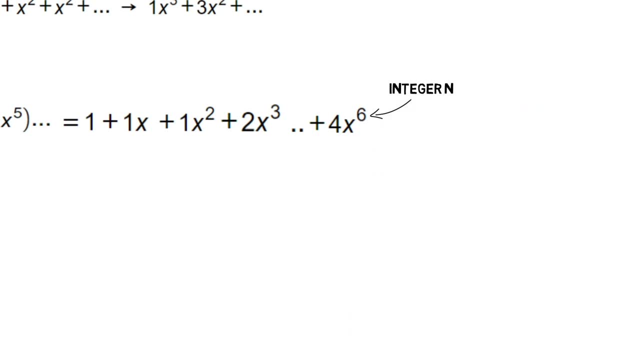 Well, the exponent represents integer n and the coefficient represents the number of ways to partition that integer n as a sum of unique integers. And you can see that if you partition 6, you will see that there are four partitions that are a sum of unique integers. 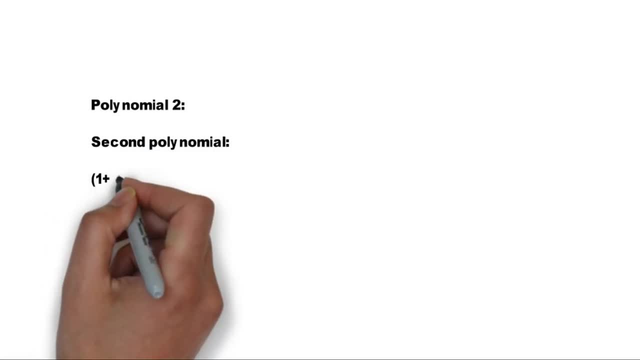 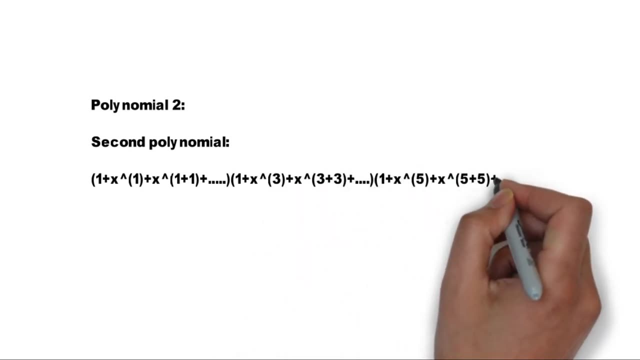 Similarly, Euler proposed that we can use a second polynomial express as 1 plus x plus 1 plus 1 plus 1, x plus cube, x plus cube plus cube, and so on and so forth, to prove that the sum of 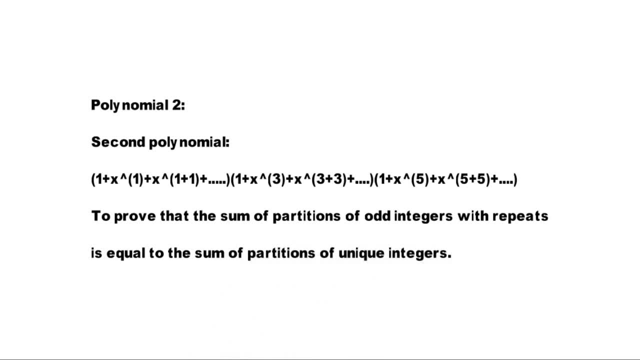 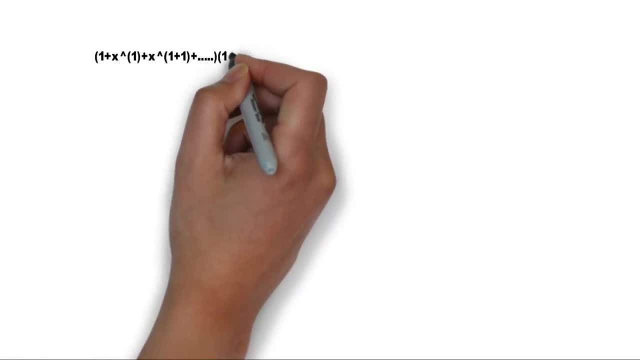 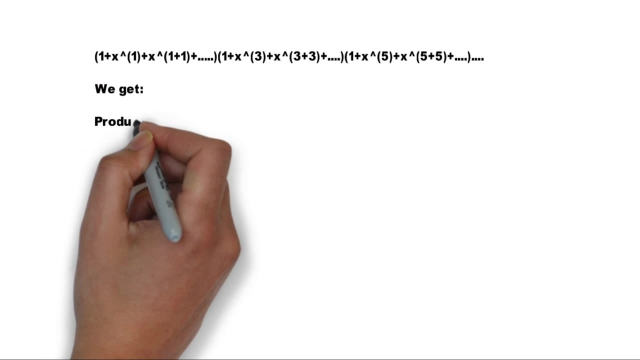 partitions of odd integers with repeats is actually equal to the sum of partition of unique integers. If we take a closer look at this polynomial and we consider taking the product of this infinite polynomial, we realize that we can actually get those partitions out of those of this polynomial. 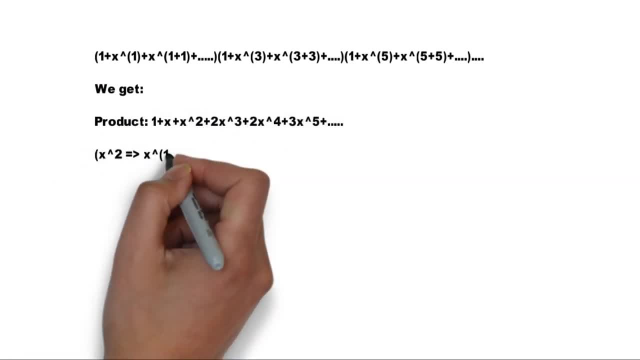 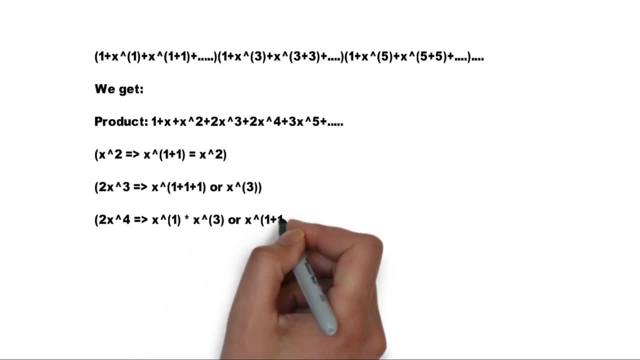 such that there is one way to get one, one way to get x, one way to get x squared, two ways to get x to the cube, two ways to get x to the 4th and two ways to get 2x squared and 2x squared. 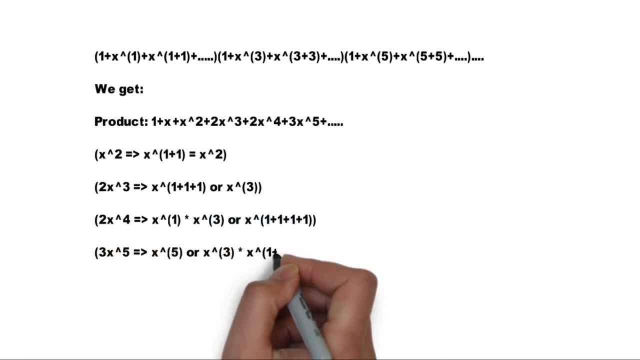 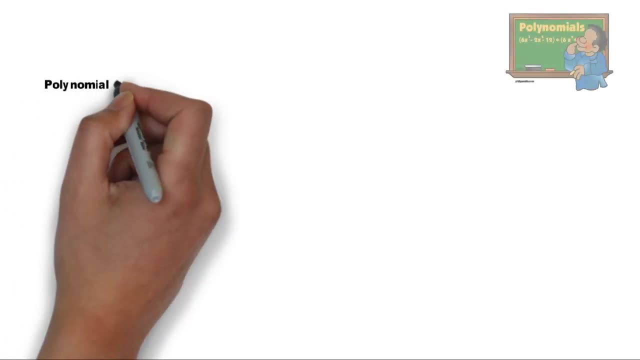 ways to get x, three ways to get x to the 5, basically, where the exponent is the number that we're evaluating and the coefficient is the actual number of partitions that you can get from that number. So how do we go about proving that polynomial 1 is actually? 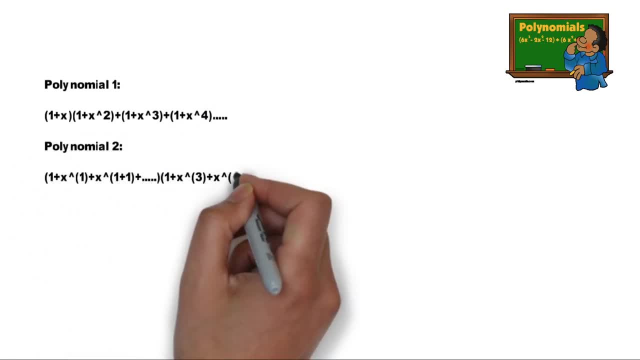 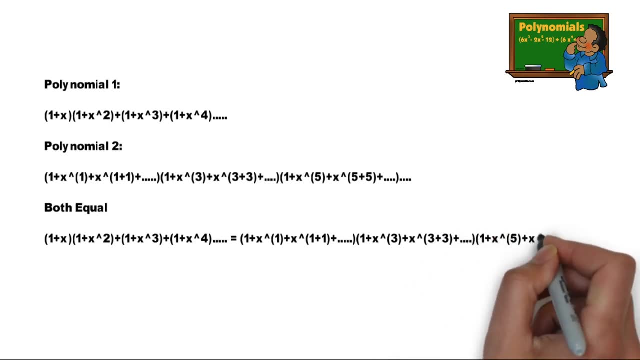 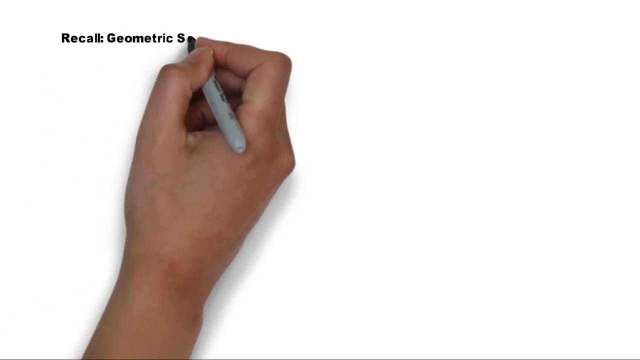 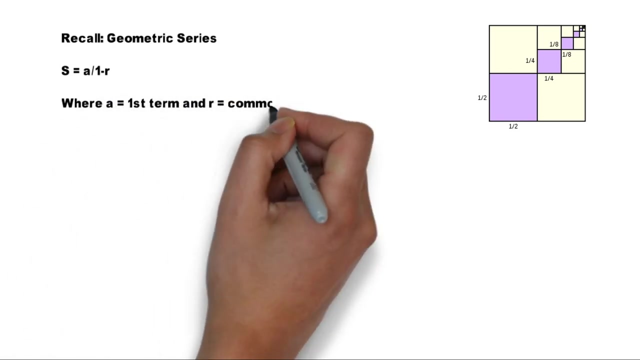 equal to polynomial 2, as Euler's theorem clearly stated. To prove this interesting fact, we can recall a geometric series which can be represented as: s equals a over 1 minus r, where a is the first term and r is the common ratio. Using our second polynomial, we can actually: 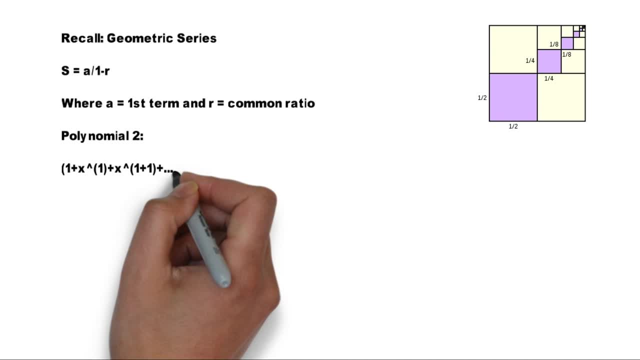 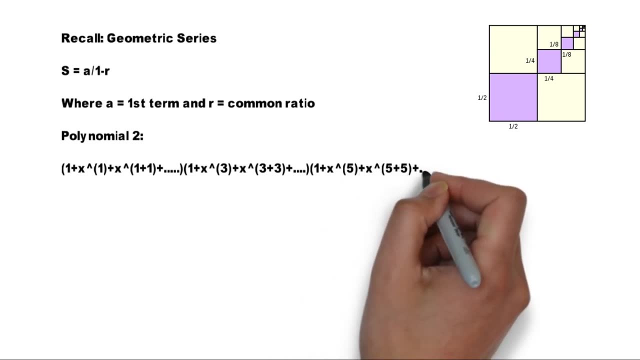 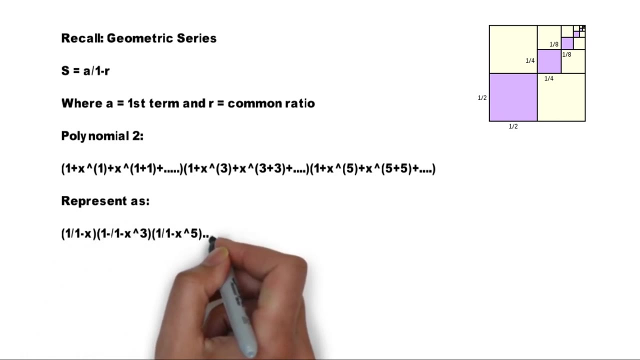 write this as a geometric series Where 1,, as you can see, would be our first term and our common ratio would be x, then x cubed, then x to the 5th, then the next one would be x to the 7th, x to the 9th and 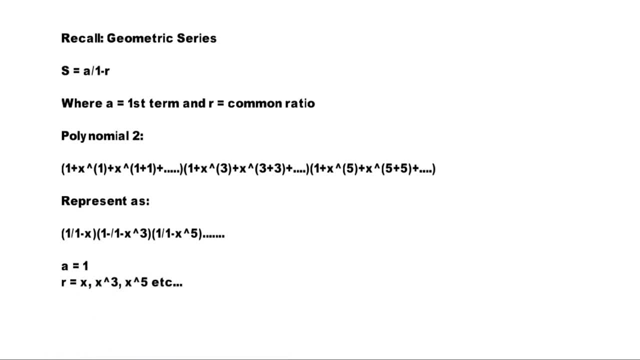 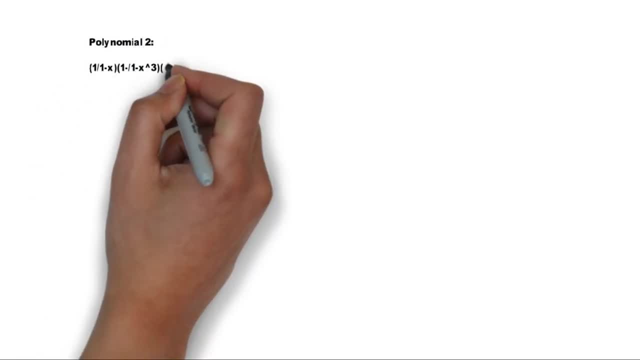 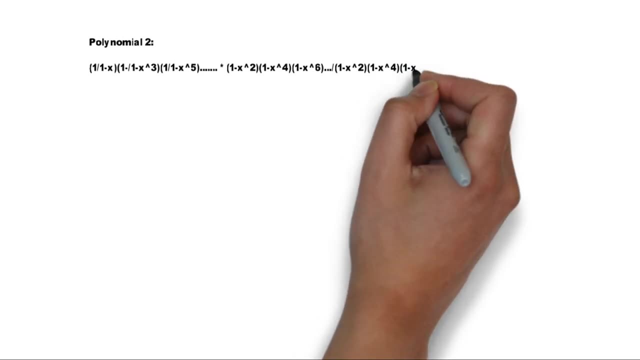 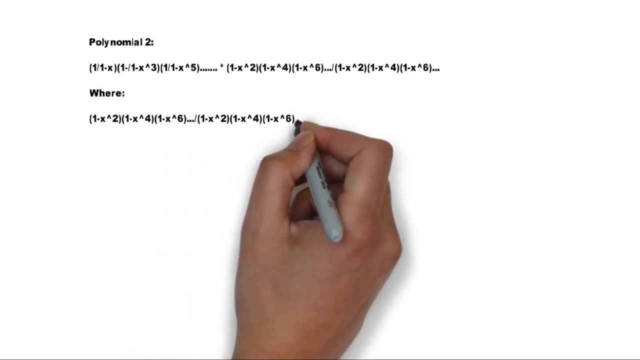 so on and so forth. Using this polynomial in its geometric form, we can then multiply it by 1, a difference of squares expression which we can actually expand out to be 1 minus x squared, 1 plus x squared, and so on and so forth. and when we actually cancel our polynomial and this, 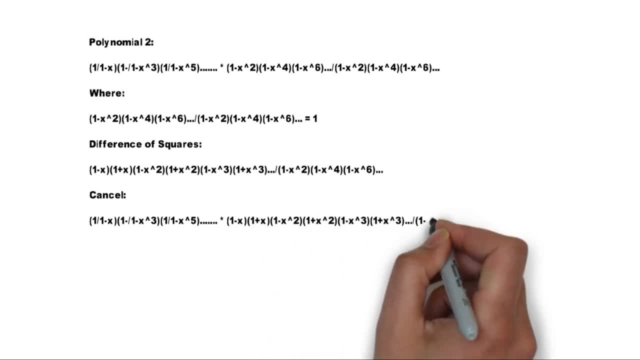 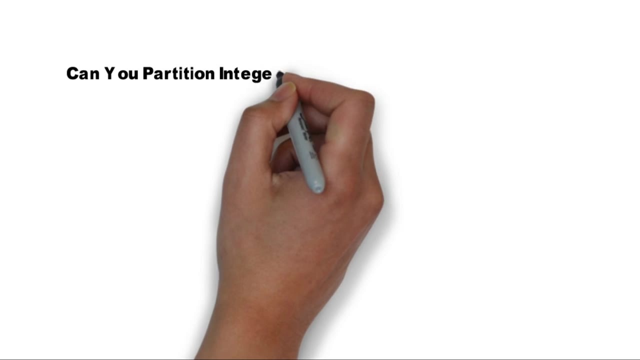 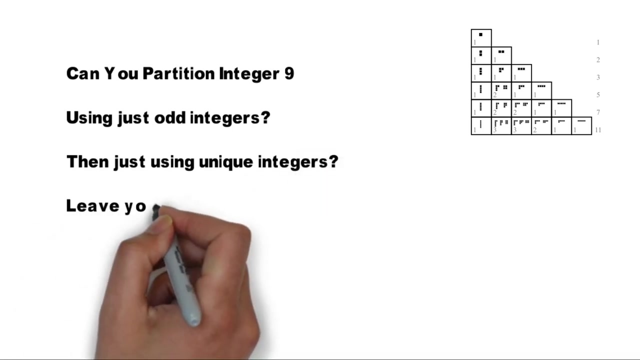 expression, we will end up getting back the exact same polynomial 1 that we had originally before this polynomial 2, which proves that the two are indeed equal. having said that, now can you partition integer 9 just using odd integers and then just try it using unique integers as well? leave your comments in the comment section below and.